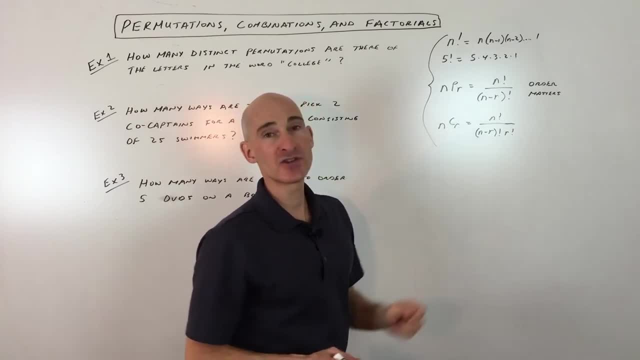 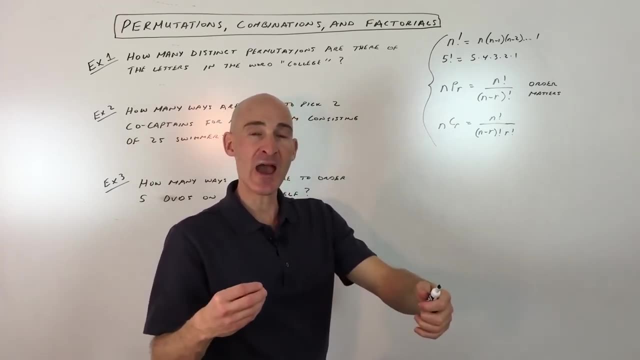 Now with permutations and combinations. what you want to pay attention to is whether the order is important or the order is not important. So, for example, if you pick two things out of a hat, and if you pick a first and then b, or b first and then a, if the order 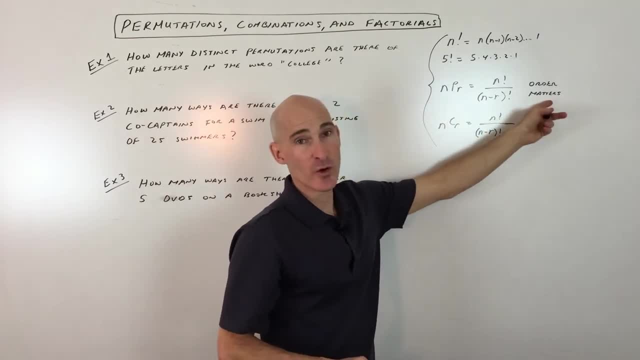 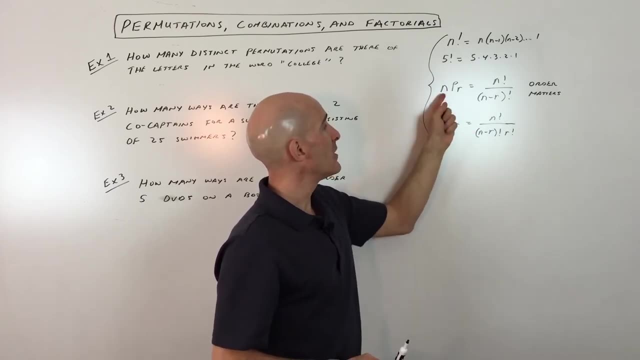 is important, then you want to use the permutation formula. If the order doesn't matter, then you want to use the combination formula. and basically what these formulas tell us are that, out of n objects, how many ways are there to pick groups of r? So, for example, if there's 10 objects, 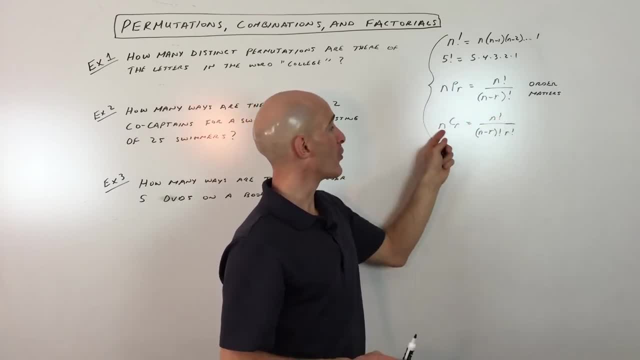 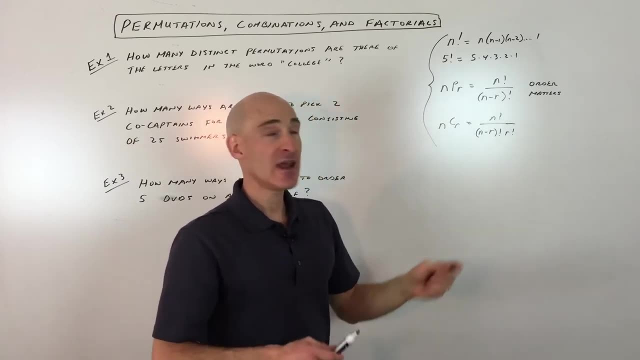 how many ways are there to pick two of them where the order matters? or out of 10 of them, how many ways are there to choose two of them where the order really doesn't matter? So a and b, b and a, that would be considered two different outcomes for permutations, but just one outcome. that's the. 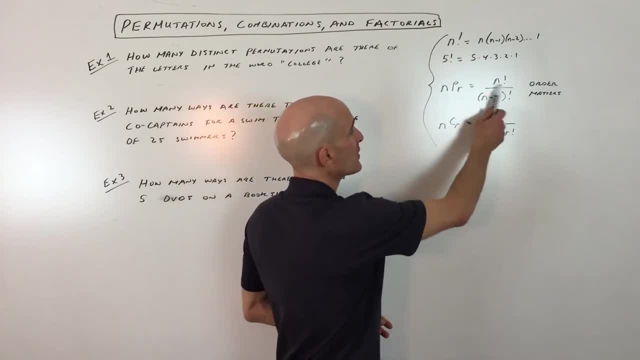 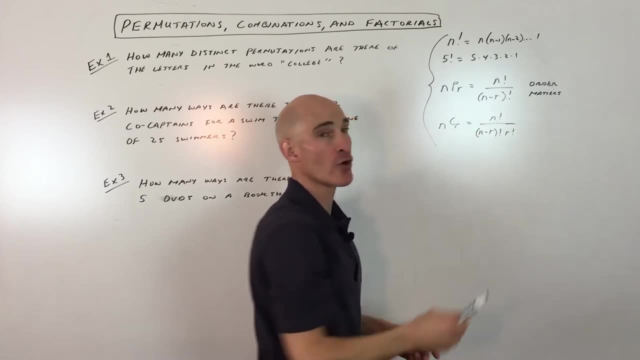 same outcome for combinations. So here's the formula here: n factorial over n minus r factorial. One is almost exactly the same except for, you can see, we're dividing by another r factorial, because we're dividing out the multiplicities. So you know, a and b, b and a, that's the same thing. 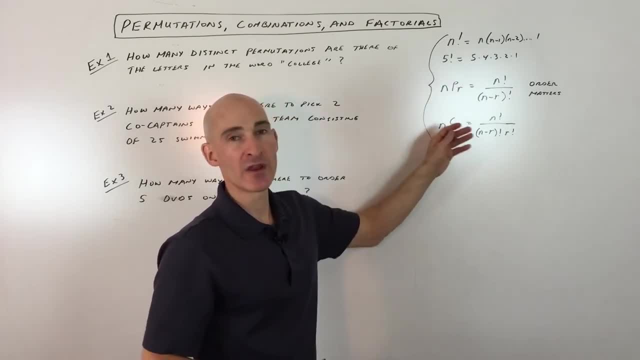 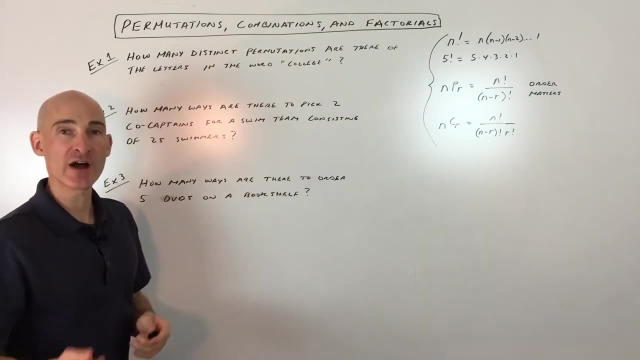 we're dividing out those duplicates, So hopefully you covered this a little bit in your math class. but just a quick review here. Let's do some examples to clear it up a little bit further. See if you can do these on your own. pause the video and then we can go through them together. 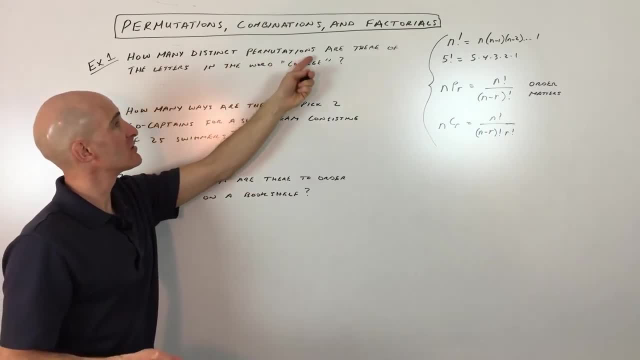 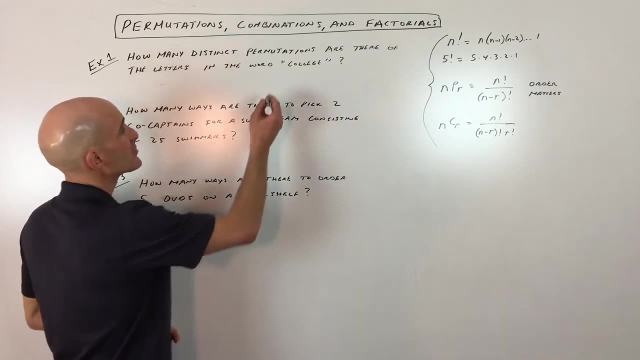 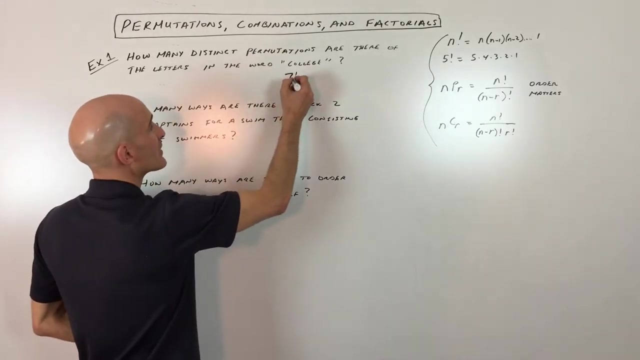 But example one says how many distinct permutations- okay, that means orderings, right- are there of the letters in the word college. Okay, so the first thing we want to look at is: okay, here's college. So college is basically one, two, three, four, five, six, seven letters. Well, there's going to be seven factorial ways of 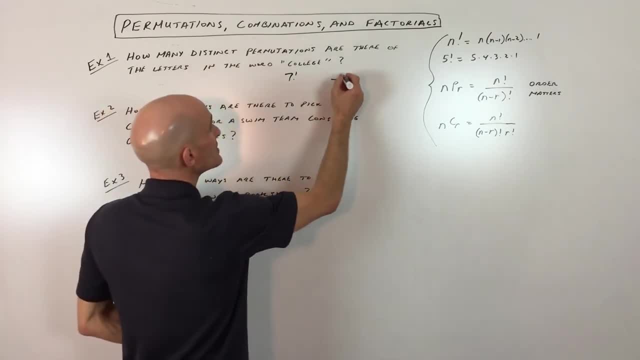 ordering seven letters. right, because you could have you know seven choices for what letter you put in the first position, and then there would be six left for which to choose for the second position, all the way down to one for the last position. So that's seven factorial. 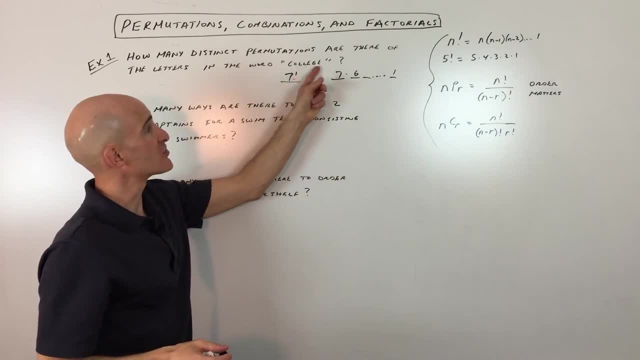 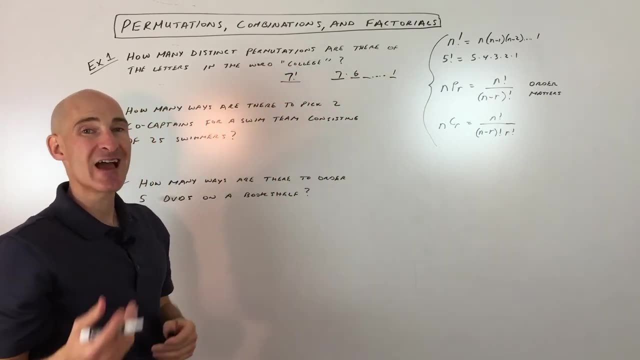 but we have a little hitch here in the sense that there's two l's and there's two e's. So whether you put these l's like this or like this same thing with the e's, if you interchange your positions it's not going to look like a different word. So what we have to do is we have 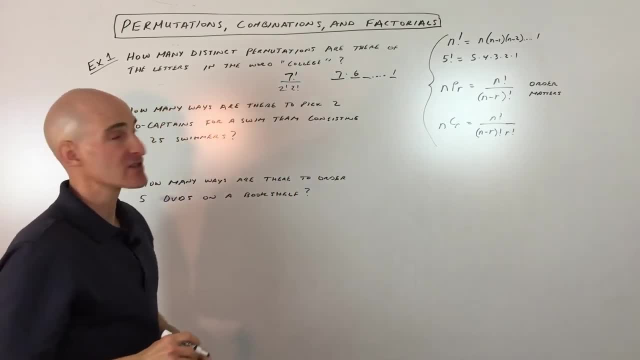 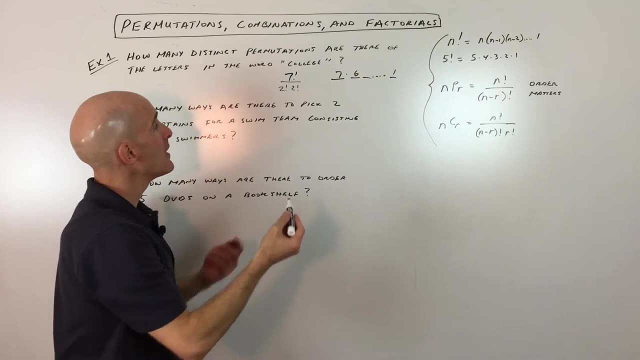 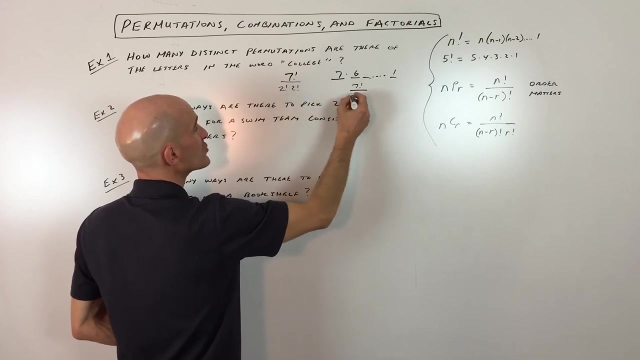 to divide out those duplicates. Now, if there was three l's, we'd be dividing out three factorial. If there was, you know, five e's, we'd be dividing out five factorial. So if we simplify this down, we get seven factorial, which is seven, six, five, four, three, two, one over two factorial, which is: 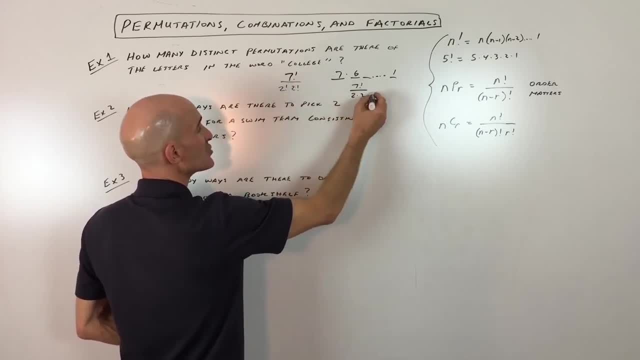 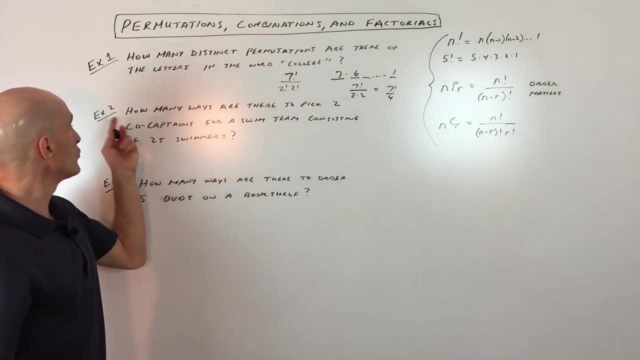 two times one, which is two, and two times one again, which is two, That's four. and we have seven factorial divided by four and you can simplify from there. So for example, two: it says: how many ways are there to pick two co-captains for a swim team? 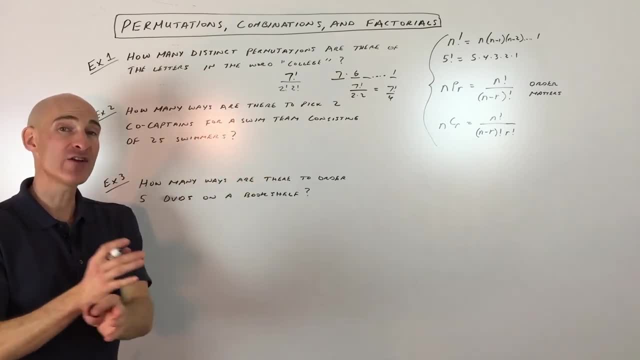 consisting of 25 swimmers. Now let me ask you a question. Does the order matter? Not really. It's not like one's like the president and one's the vice president. You know they're on the same level, They're co-captains. So in this case, we're going to use the combinations and we're going to 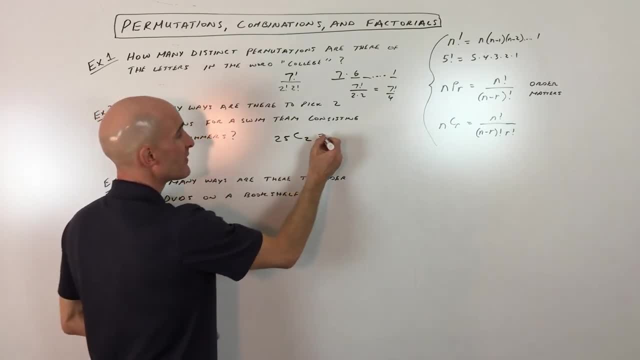 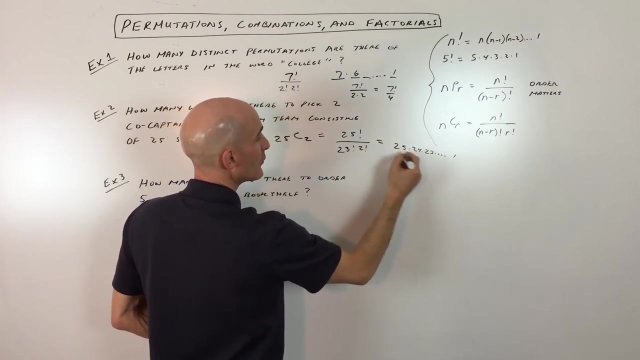 see how many ways are there to choose two where the order doesn't matter. So if we simplify this, we get 25 factorial over 25 minus two, which is 23 factorial, two factorial. Now, if you want to simplify further, 25 factorial is 25 times 24 times 23, all the way down to one: 23 factorial is 23. 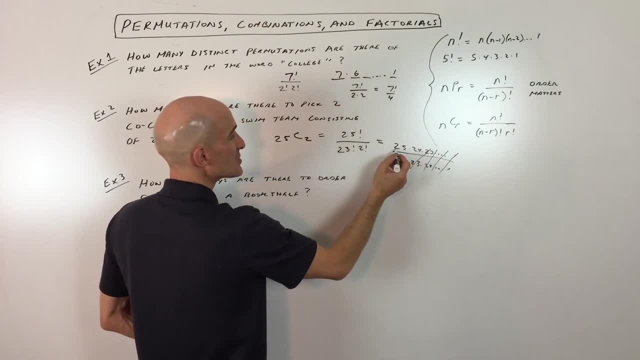 times 22, all the way down to one, And you can see those are canceling. So you just have 25 times 24, all divided by two times one, which is two, And then you know you can simplify it all the way down. 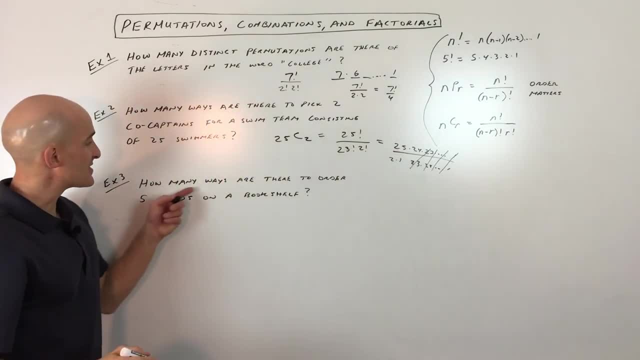 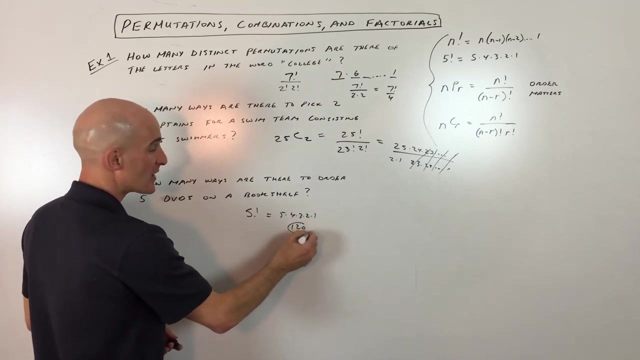 Simplify it from there. Okay, now example three. it says how many ways are there to order five DVDs on a bookshelf. Okay, this one's pretty straightforward. It's just going to be five factorial, which is five times four times three times two times one, which is 120 different. 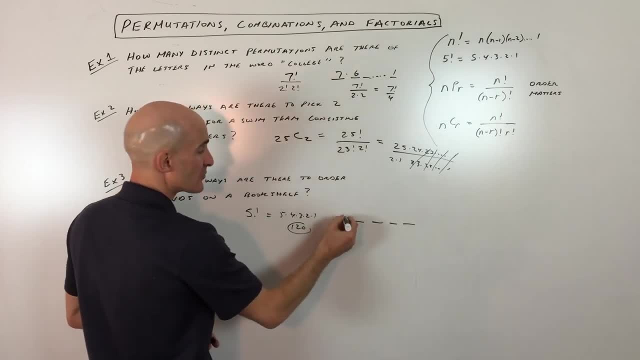 ways, And you could diagram it out like this: There's five choices for which DVD you put here, and then now there's only four DVDs left to pick for the second position, all the way down to one. Multiply those together and you get 120. 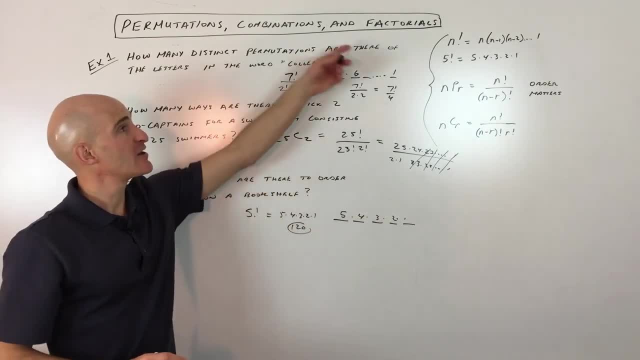 So a review here of permutations, combinations and factorials. You might want to memorize those formulas, so it makes it a little bit easier when you're, when you see these types of problems on the test.